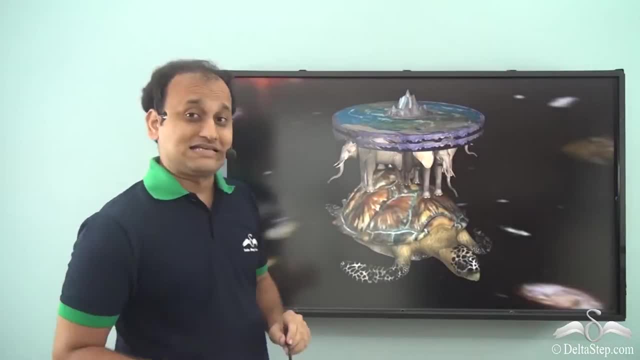 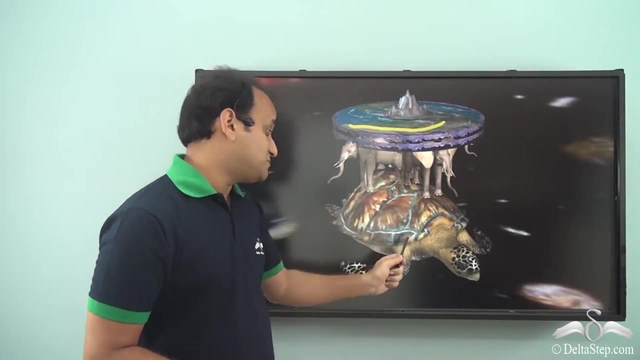 In fact, some ancestors believed that our flat-surface earth is actually being held in the space by a giant tortoise. Well, all this we imagination control displays that these market. There is an information: the wearings of payments were made by their prices. pur triple sense of. 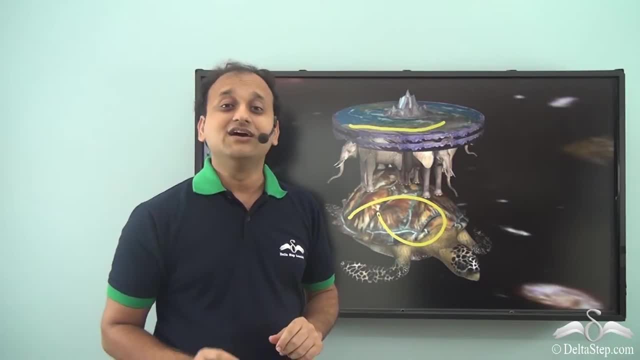 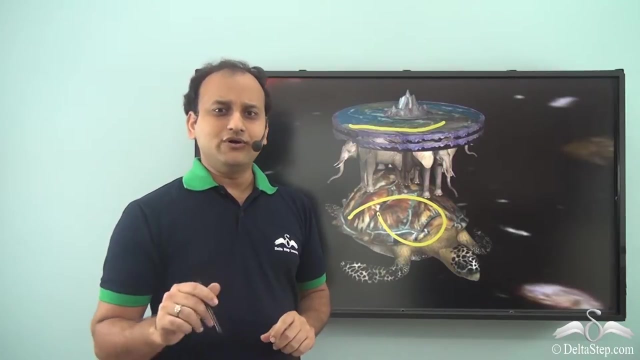 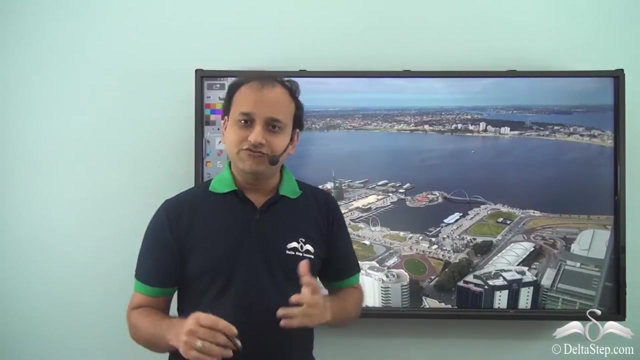 imagination of us humans because we did not understand the true nature of our planet Earth. So now we have a lot of gadgets and space stations and rockets and aeroplanes, so we can now understand better the actual nature of our planet Earth. So let's observe what we see on our planet Earth's surface. If you see the 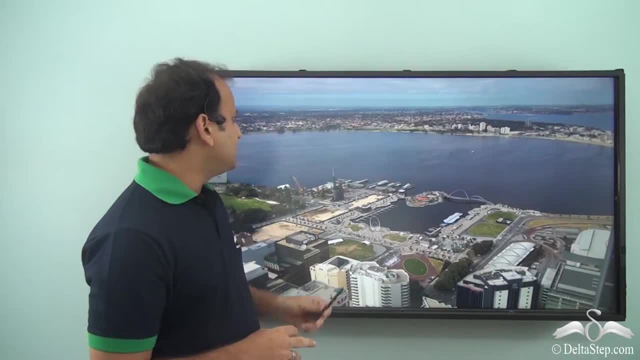 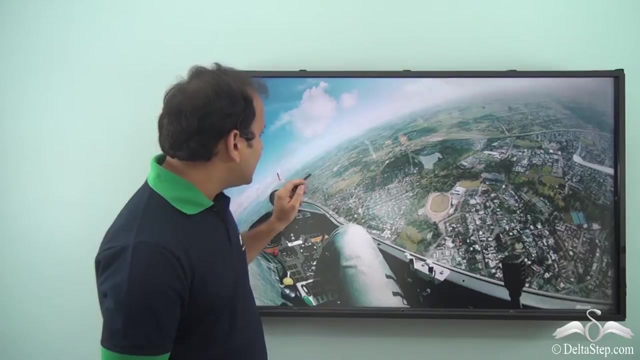 Earth's surface from your, say, terrace. it would be something like this, which looks pretty flat, isn't it? Now, let's move a bit higher Now. from an airplane which is taking off, you could see that actually there is some sort of a curve, isn't it? 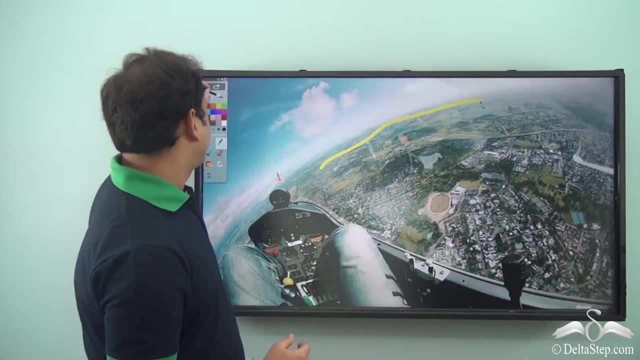 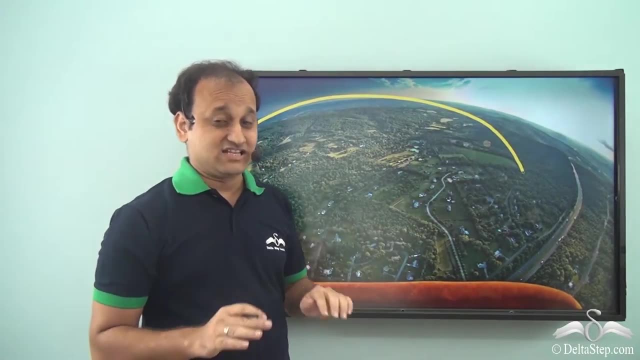 Let's move a bit more higher on an air balloon- Now this looks much curvier. Now let's move a bit more higher on an air balloon- Now this looks much curvier. So what we were seeing as flat from our terrace, now from the air balloon, looks. 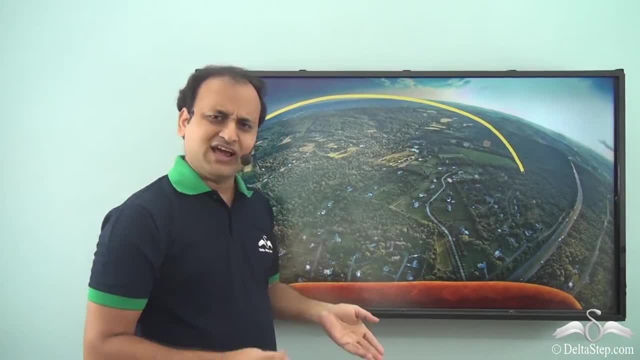 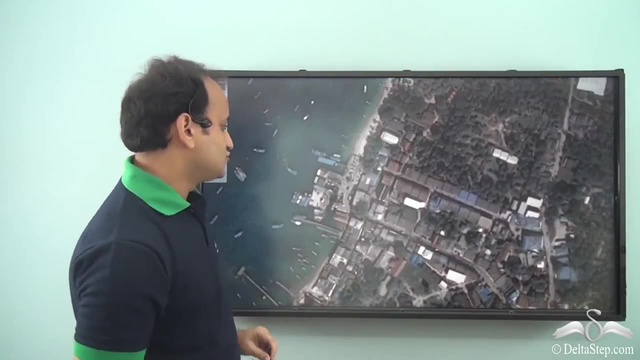 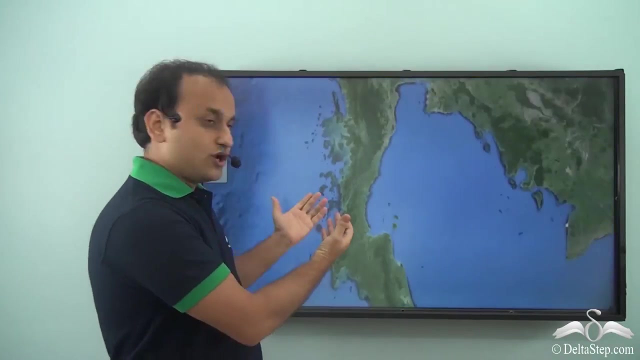 much curvier. So just now it was flat and now it looks curvier as the height increased. Let's see one more level up. So this is a flat Earth and now we are zooming out of it, that is, we are moving away from that place into the space. So 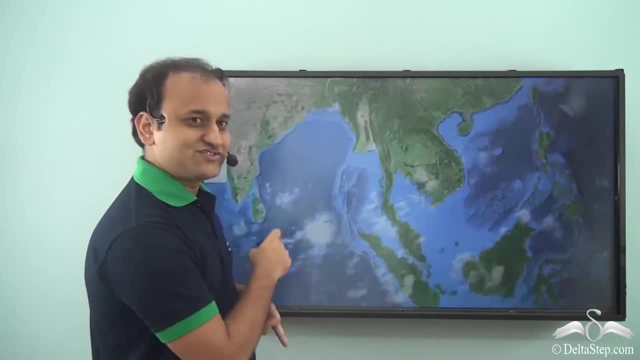 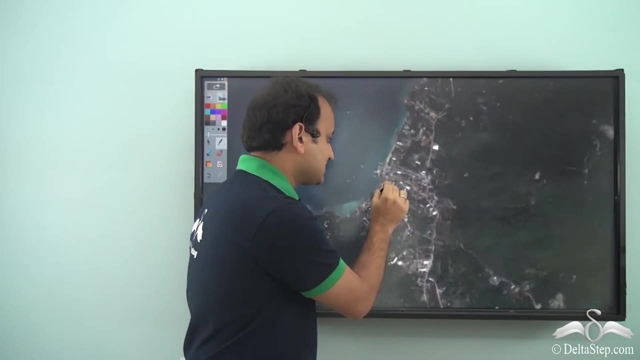 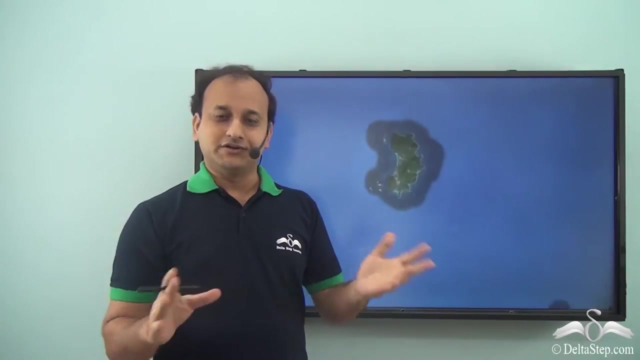 as we are moving away. what's happening? you see? You see the Earth is round and then, when we zoom in again and we go to that particular place, it is flat. So what exactly is happening? Well, our Earth, as you can see in this, 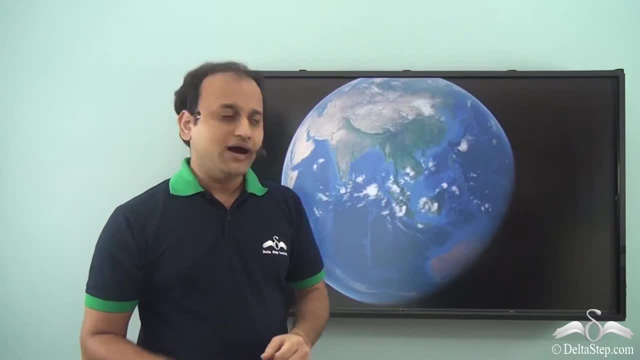 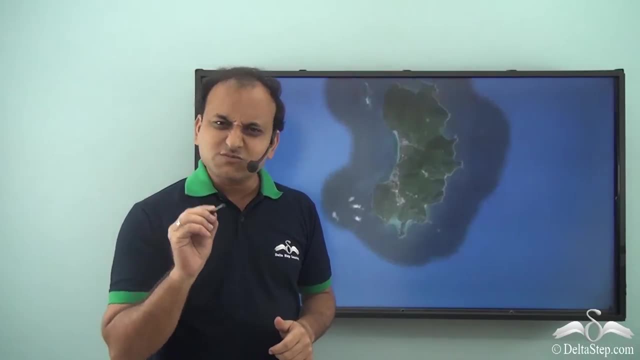 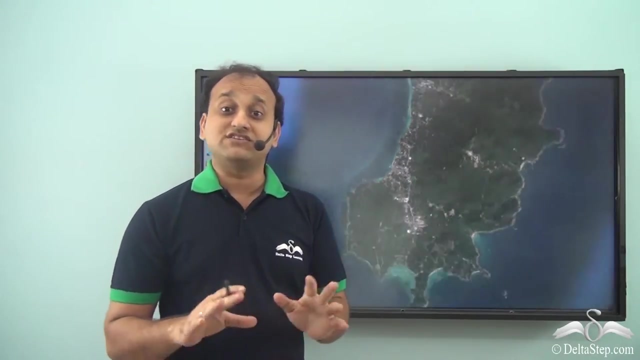 particular animation is round, But we are very small as compared to this huge Earth and that is why we can only see a very small area of that big ball of Earth, And because of that you see that particular surface as flat. Well, something else will make it clearer. 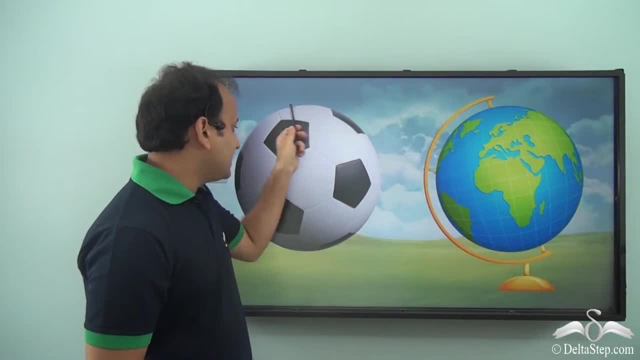 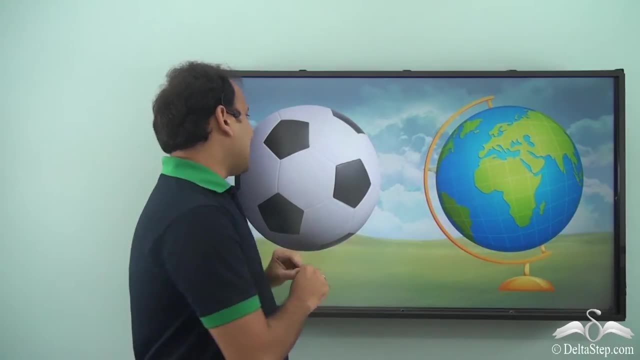 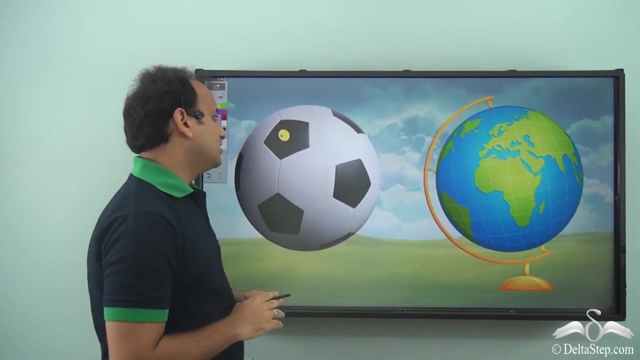 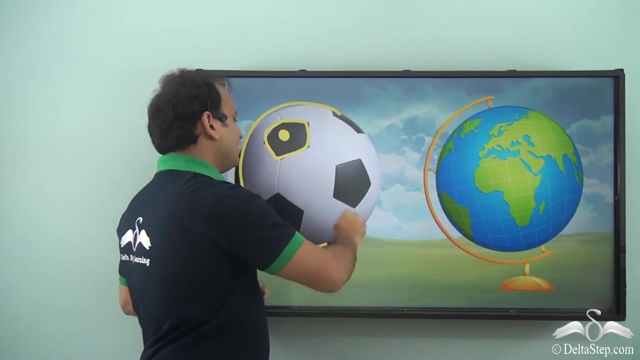 See. our Earth looks something like this football or a globe, if you have seen one in your geography lab. So our Earth actually is something like this. Now, if an ant stands here, for it this will look like a flat surface, because this is a huge ball for that. 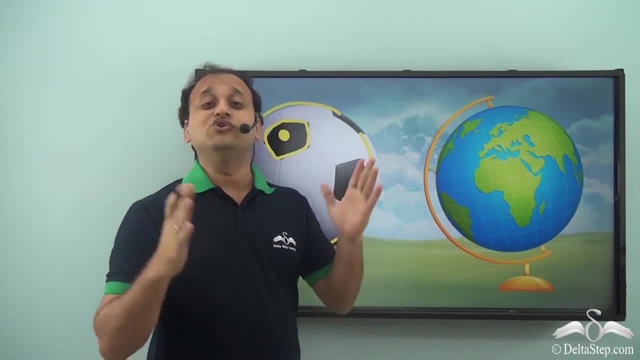 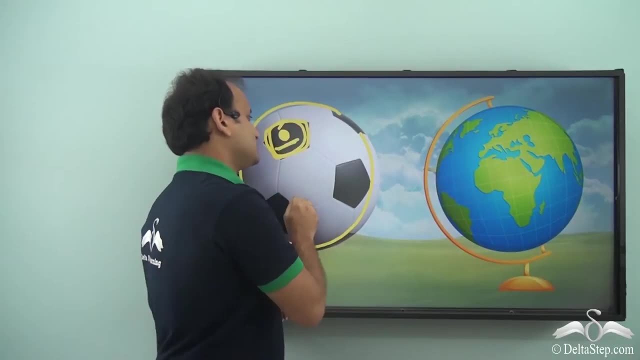 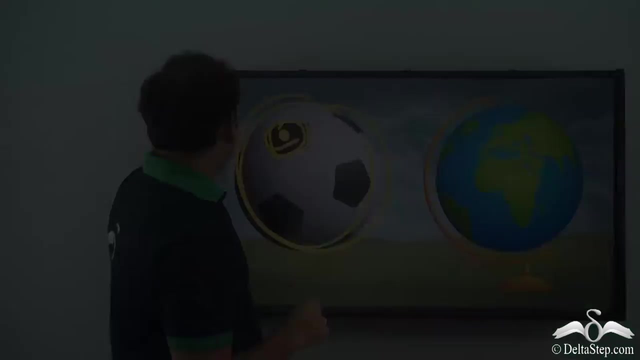 small ant. So we are like that ant on the huge ball of Earth, and that's why we can only see a small area of Earth which looks flat to us, But if we move out in the space we see the whole ball which is actually round. So this is how our Earth. 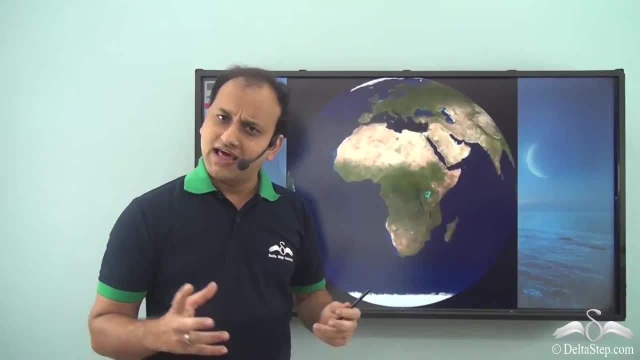 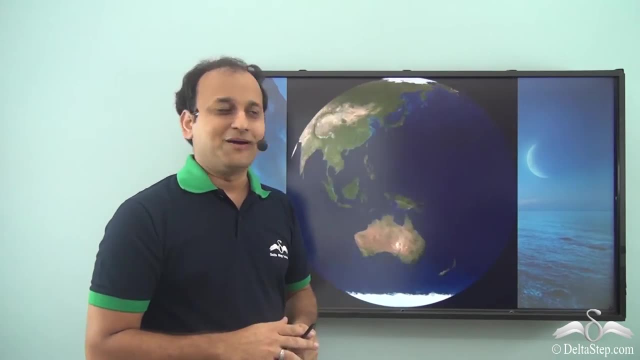 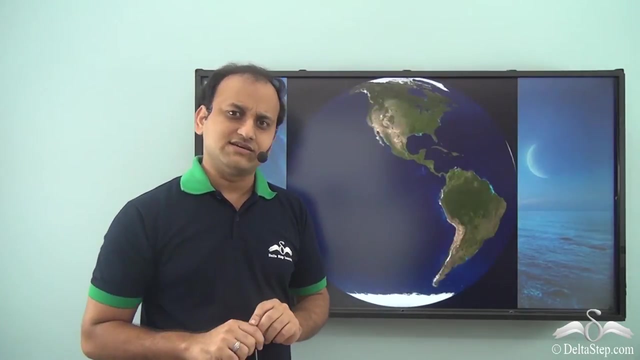 looks from space, Which is roundish like a ball, And this is how it looks from a satellite or, if you look it, from a moon, But as we live on it, we are not able to see this true nature of our planet Earth. Now the question arises that if it is round and 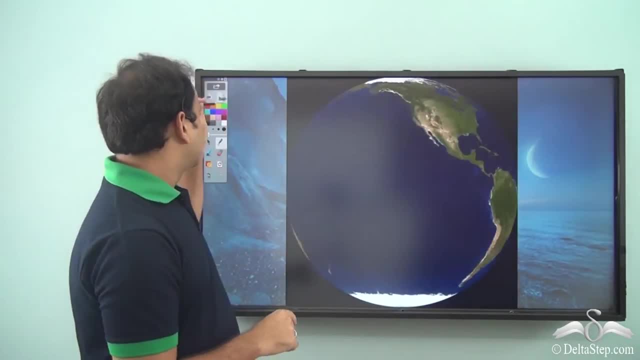 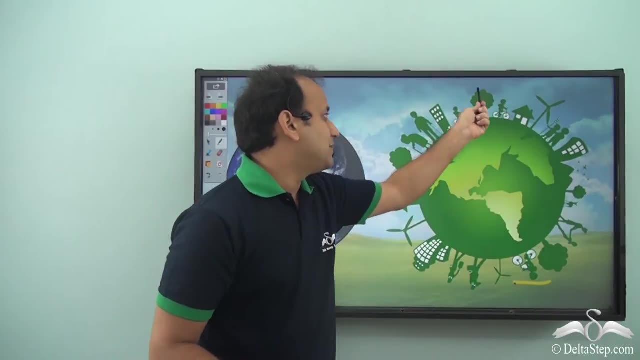 we are living on it, then why don't we fall from it? See, we are living on the planet Earth like this. Now, some people are on this side, some people are on this side, and some are even here and here, So why don't they fall off from the planet Earth? 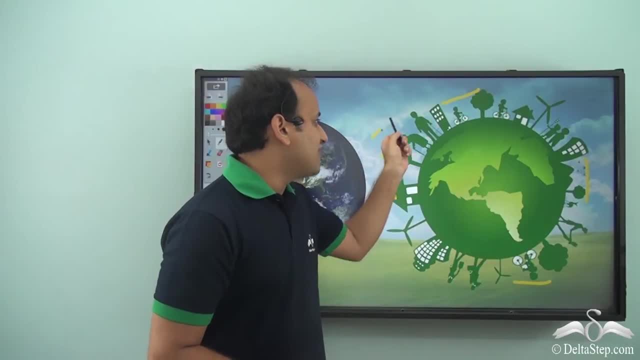 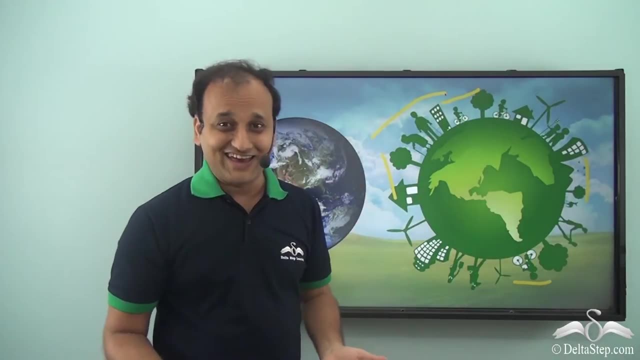 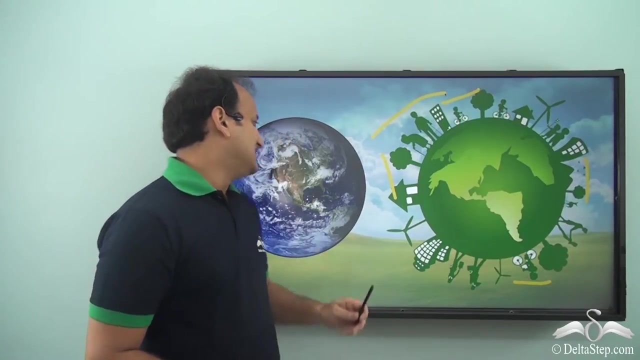 That is because our Earth holds everything like a magnet, and that is why everybody is able to go about their jobs without really thinking that which side of the Earth they are and will they ever fall down from the planet Earth? So this is how our Earth looks like, and it holds us like a magnet. 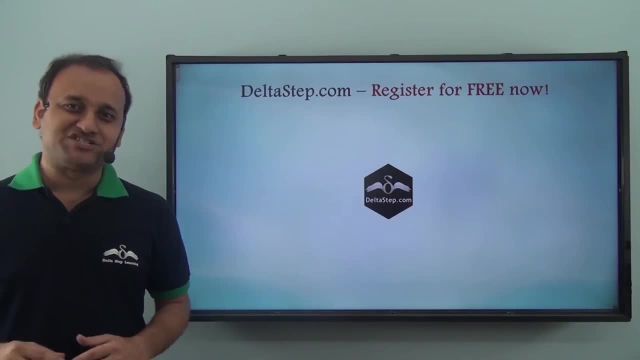 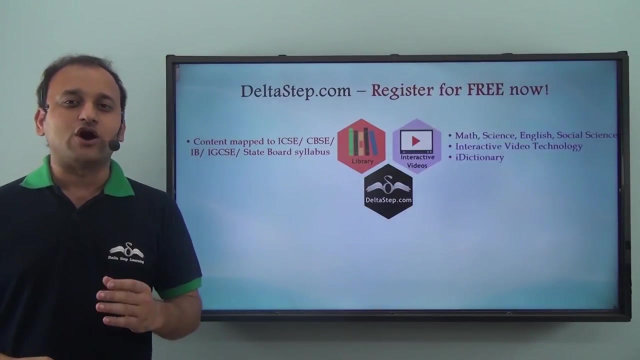 Don't forget to subscribe to our channel. You can also register for free at deltastepcom to get all learning resources as per ICSE, CBSE, IB, Cambridge or any other curriculum. Over 5000 amazing lectures across Maths, Science.